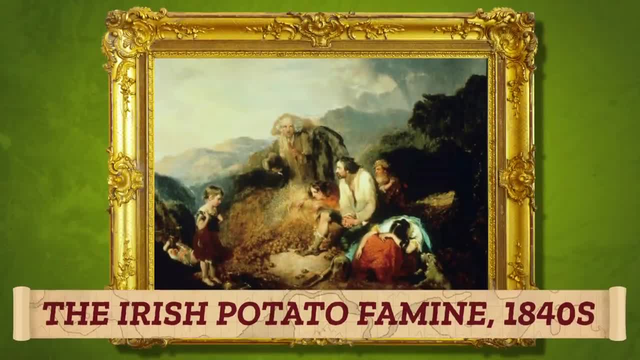 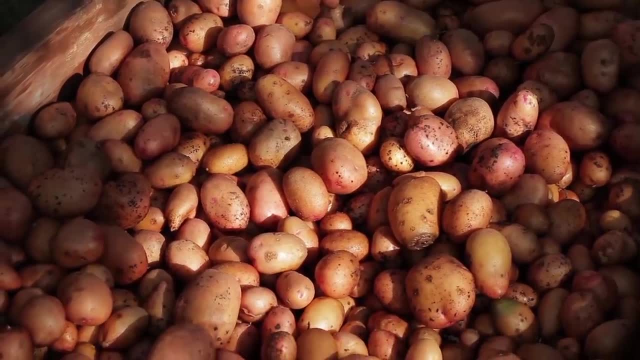 what were we talking about? The potato has many claims to fame around the world, from the devastating Irish potato famine of the 1840s to the salty magnificence of French fries. But this humble tuber originated neither in Ireland nor France. It was domesticated- the process of adapting plants and animals. 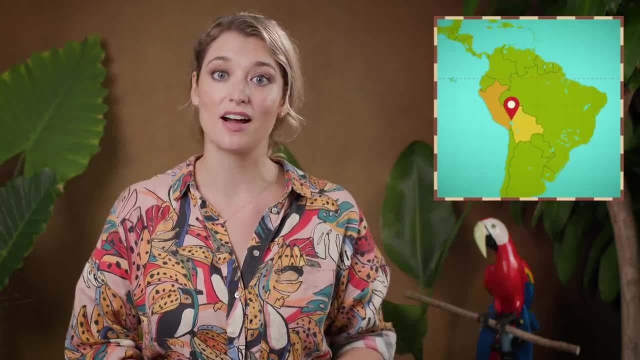 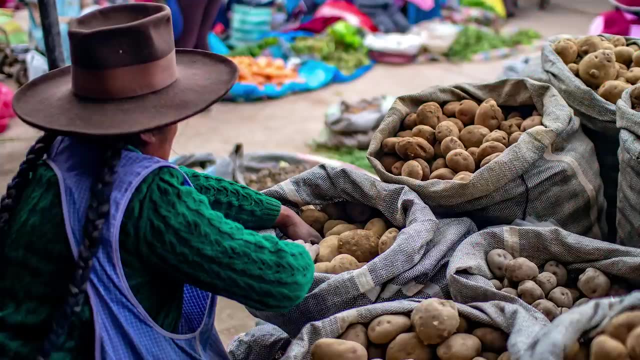 for human use about 7,000 to 9,000 years ago, near Lake Titicaca, now on the border of Bolivia and Peru, in the central Andean highlands, where it's known as Mama Jatha, the mother of growth. 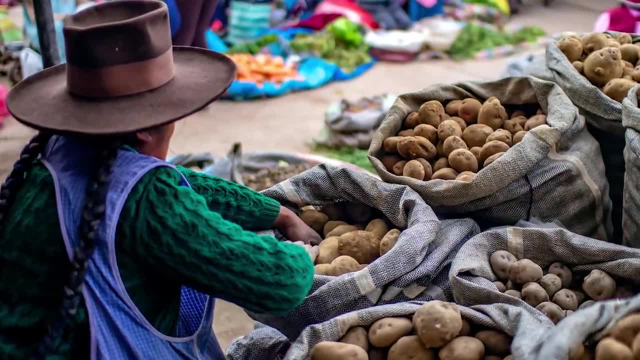 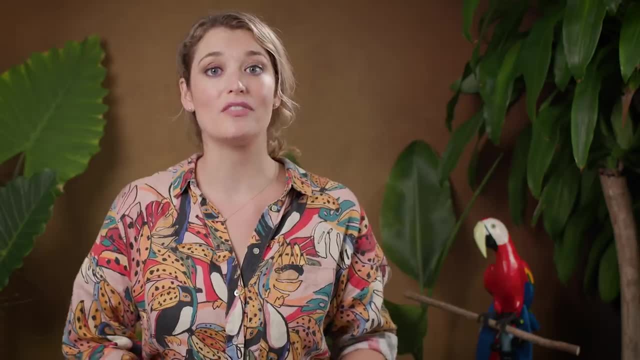 So, as geographers, we ask: why were potatoes domesticated here and not anywhere else? The story involves the ideal conditions needed for growing potatoes, how climates change across space and the ingenuity of the Andean farmers. So today we're going to go bananas. 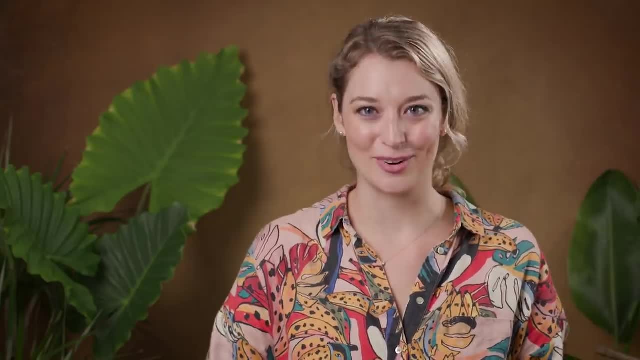 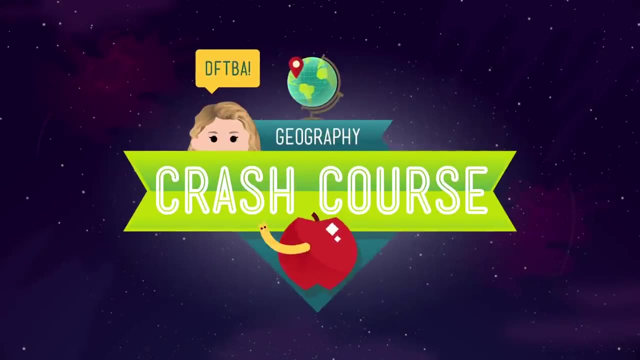 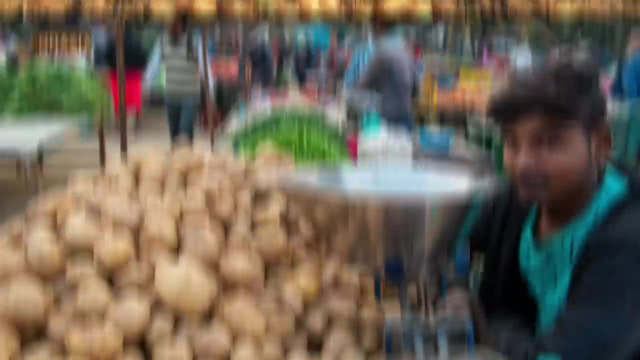 about potatoes. I'm Alizé Carrère and this is Crash Course Geography. Worldwide, the potato is one of the most calorically important food crops. along with corn, wheat and rice, It's the cornerstone of food security for millions of people, Like in 2019 alone. 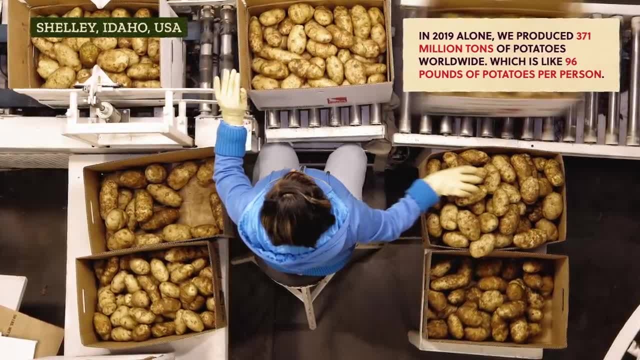 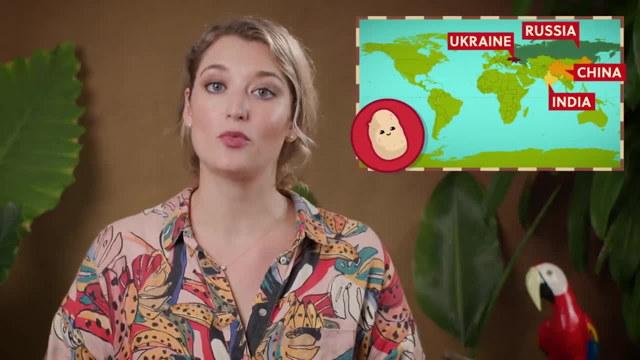 we produced 371 million tons of potatoes worldwide, which is like 96 pounds of potatoes per person. Today, the top producers of potatoes are China, China and China, India, Ukraine, Russia and the US, But potatoes are still integral to their South American. 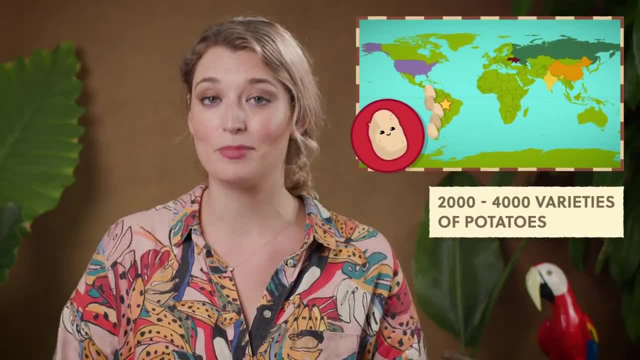 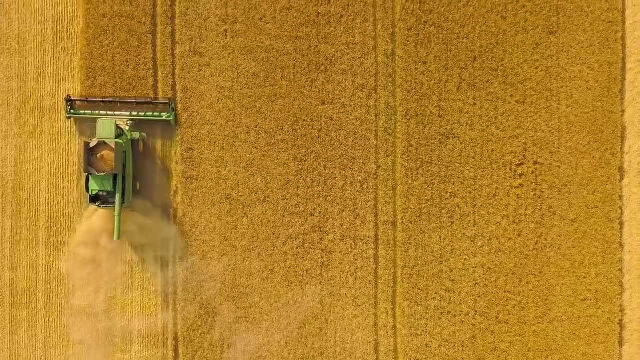 homeland. Somewhere between 2,000 and 4,000 varieties of potatoes are grown along the length of the Andes mountain chain. Different crops need different temperatures, precipitation and soil conditions to thrive, which brings us to an important distinction. we need to get to the root of our potato story. 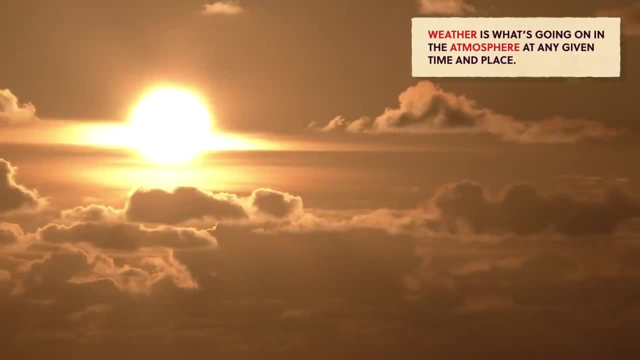 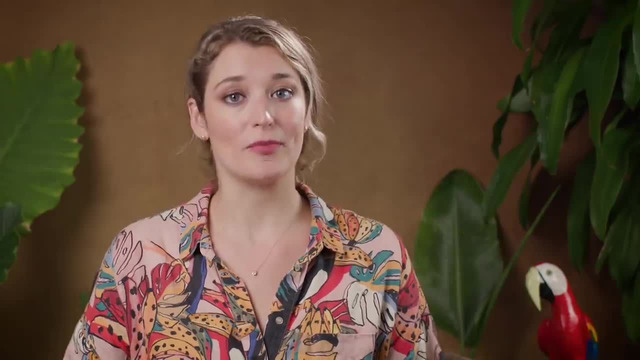 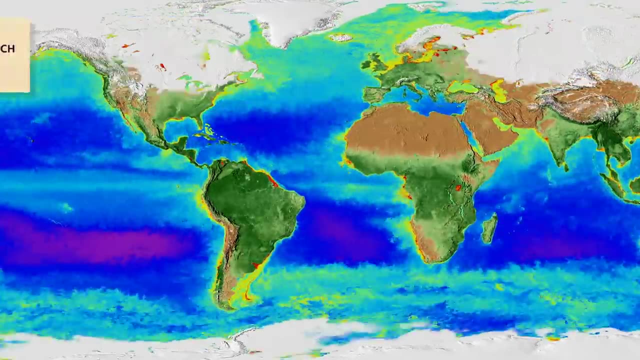 Whether it's fresh, hot french fries or cold soggy ones, weather happens in the short term and is difficult to predict. But climate is a region's average weather over many years, which is much more predictable and based on trends. So we don't know what the weather will be like in New York City. 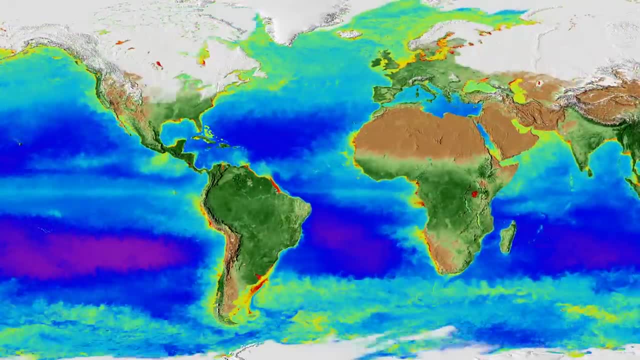 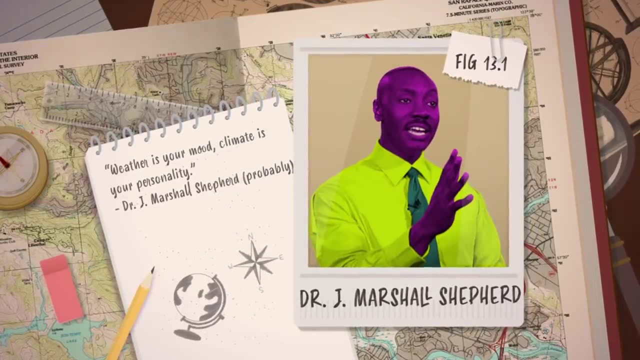 on January 20, 2025., But we do know that it's usually chilly, because New York City has a cold winter climate. It's like what former president of the American Meteorological Society, Dr J Marshall Shepard, famously- probably- said: Weather is your mood, Climate is your personality And my personality. 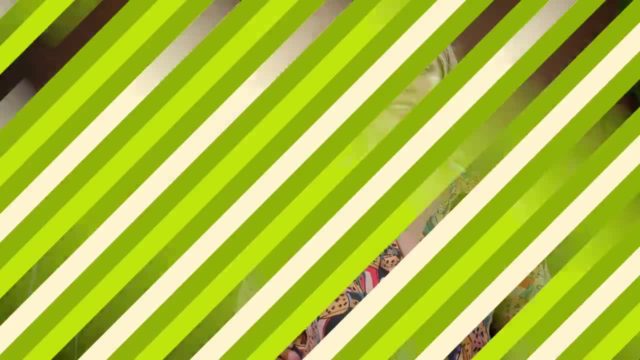 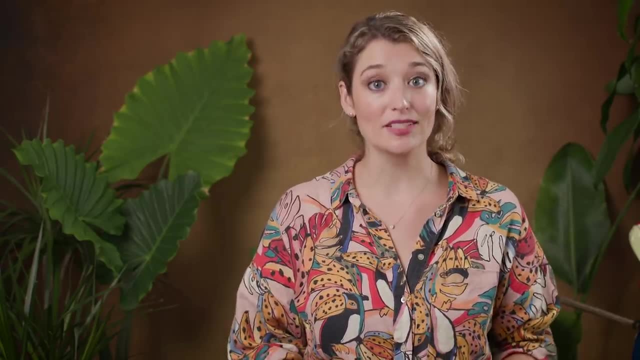 is a proud potato fan, Even though we've all had disappointing fries before, Just like there are endless human personalities based on our DNA and how we grow up. all the possible combinations of temperature, precipitation, wind and ocean currents give us a variety. 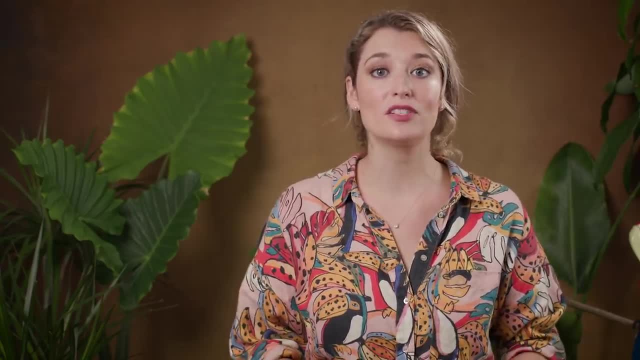 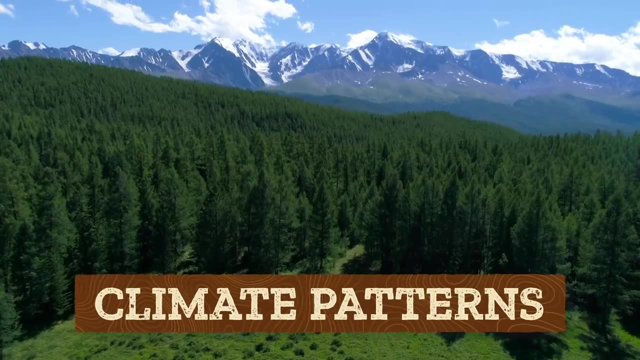 of global climates, And all of those processes begin with patterns of insulation or incoming solar radiation across the globe. For example, mountains have complex climate patterns or the somewhat predictable variation in climate. These mountain climate patterns come from the way insulation and temperature. 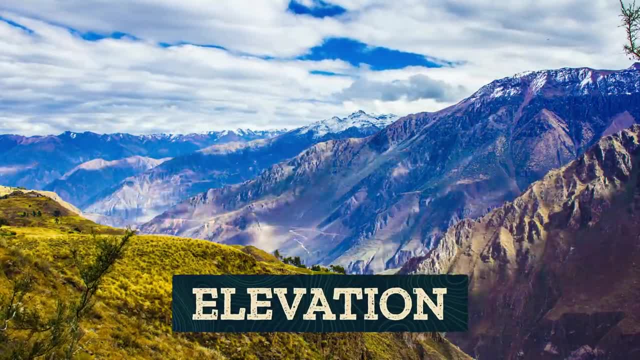 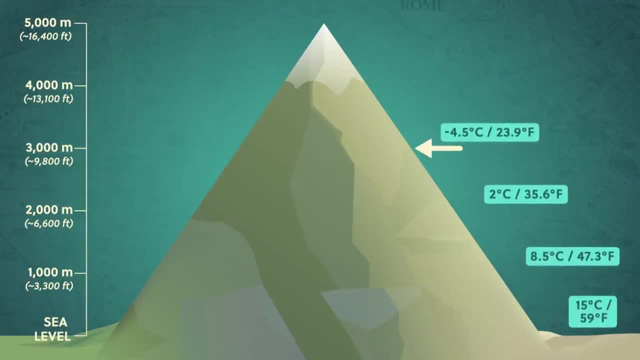 change as we go higher in elevation or the height of a point on Earth's surface above a reference like sea level. In fact, no matter where we are on Earth, for every 1,000 meters we go up in elevation, the air temperature decreases by 6.5 degrees Celsius on average, which is the normal lapse. 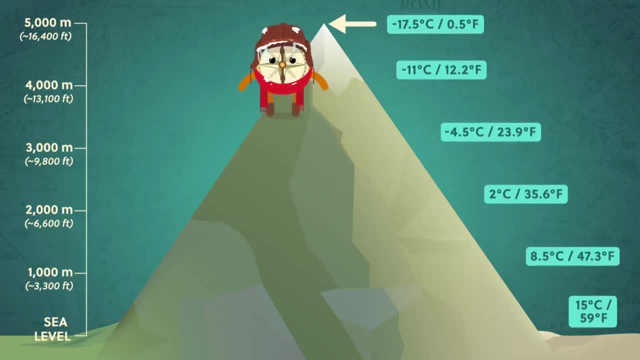 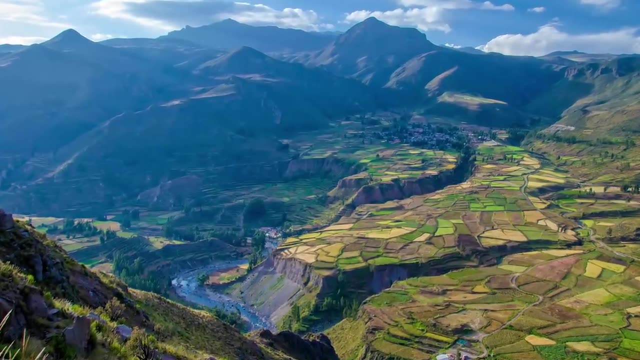 rate. If you've ever hiked or driven up from the base of a mountain, you've probably felt the air get chilly or brought extra layers to handle the cold temperatures. The normal lapse rate has big implications for Latin America's physical geography, especially near the equator. 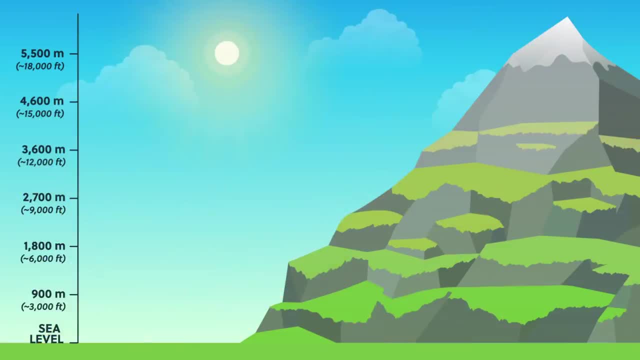 As we climb the Andes Mountains from sea level, we can define our major climate zones based on elevation that have dramatic changes in plant life. At the foot of the mountain is Tierra Caliente. Tierra Caliente, or Hot Country, a lowland zone of broadleaf, evergreen tropical rainforest. 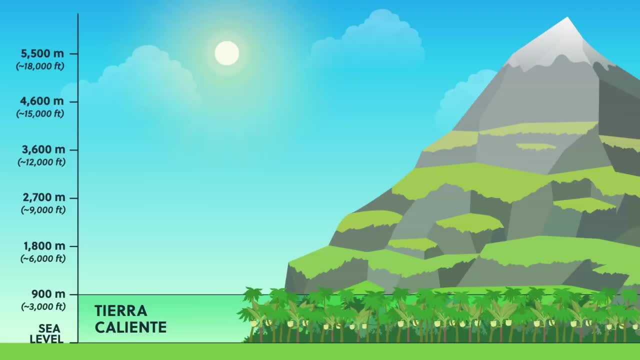 The warmth and humidity here allow extensive tall trees and a dense year-round leaf canopy to develop. At about 900 meters we begin to see mild temperate conditions and deciduous forests in the Tierra Templada. Then, as we continue our climb at about 1,800 meters, temperate conditions get chillier. 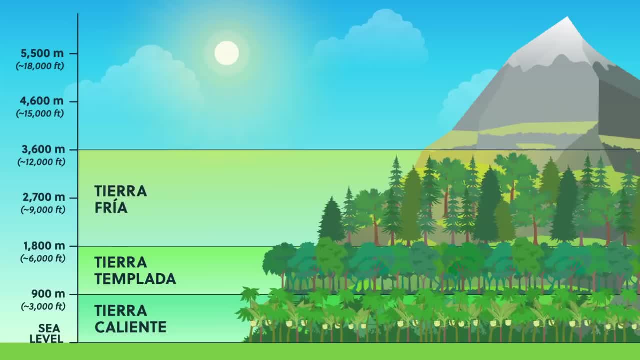 Colder temperatures and coniferous forests mark the Tierra Fría. As we move higher, each zone gets smaller And at 3,600 meters we reach the windswept Andes Mountains. We reach the windswept Tierra Helada, or Frost Country. 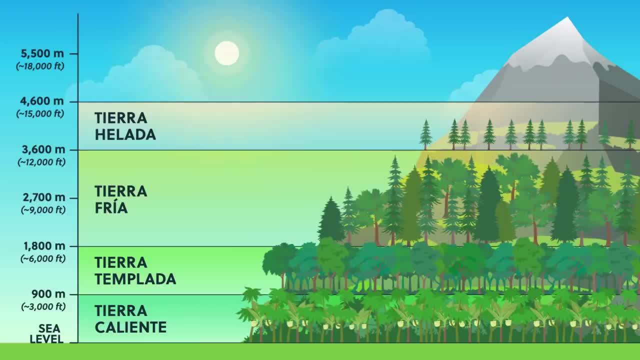 In the lower reaches of this zone, pine forests transition to alpine meadows and grasslands and mark the treeline, the upper limit of where trees grow. Further up, around 4,600 meters, we see a shift from grasses to hardy lichens and mosses. 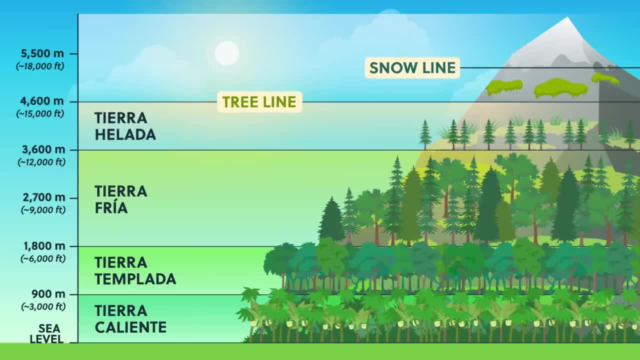 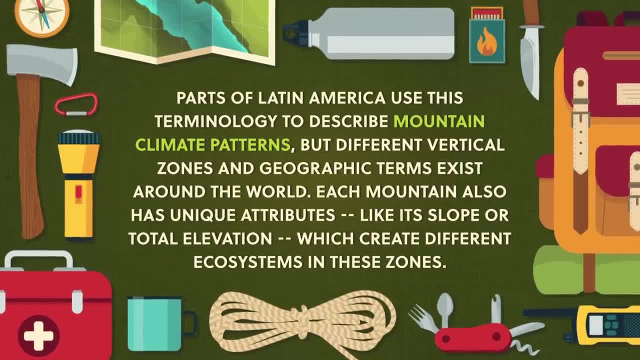 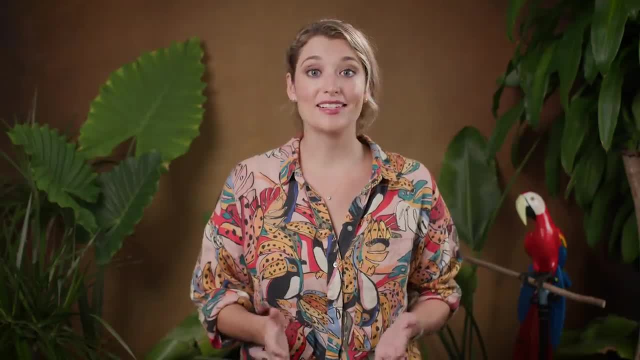 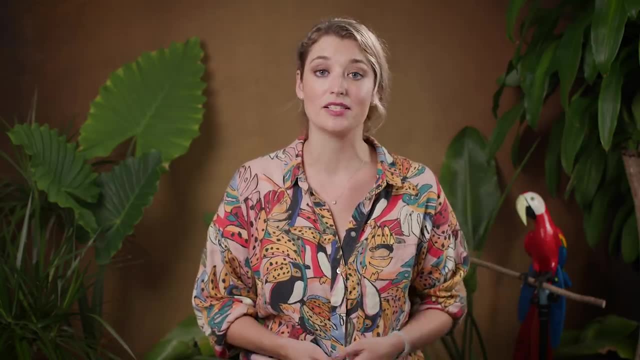 different vertical zones and geographic terms exist around the world. Each mountain also has unique attributes, like its slope or total elevation, which create different ecosystems in these zones. The process of paying attention to geographic conditions, like mountain climate patterns, and using them to answer questions like: why were potatoes domesticated in the Andes Mountains? 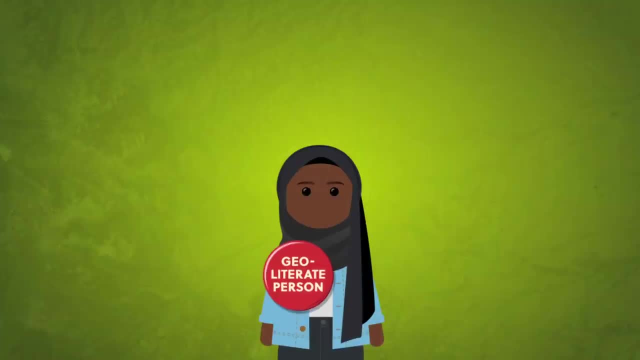 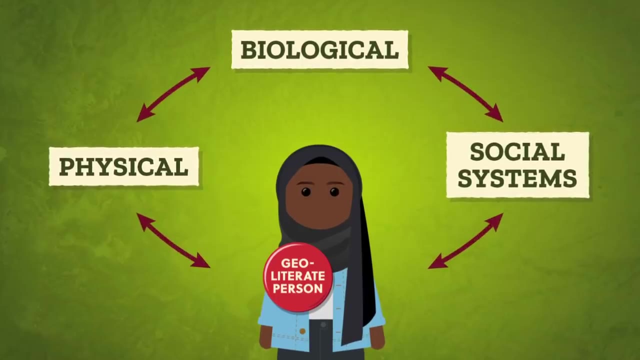 and not anywhere else, is called geoliteracy. A geoliterate person understands that the world works as a set of physical, biological and social systems and that processes within these systems are the ones that make up the world. These systems connect places to each other. 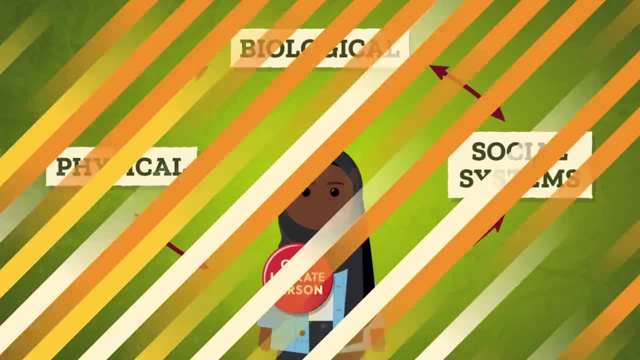 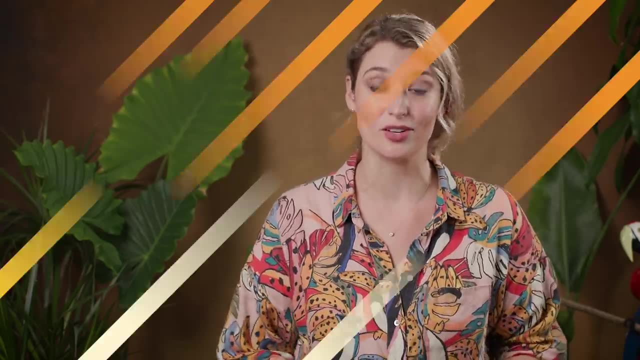 We can use these observations to interact with our environment and create particular outcomes. And even though geoliteracy might be a modern term, engaging with the world with a geoliterate lens is something people have been doing for thousands of years. Like 7 to 9 thousand years ago, Andean farmers observed how a mountain was made of spaces. 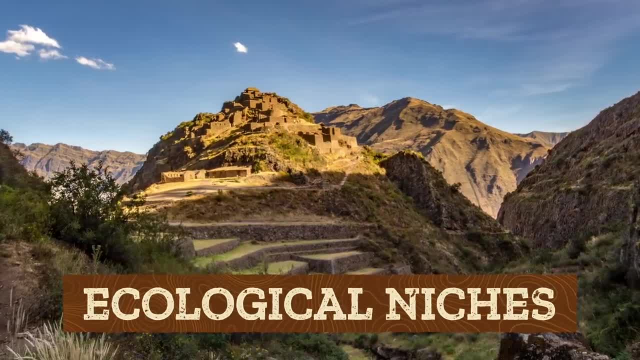 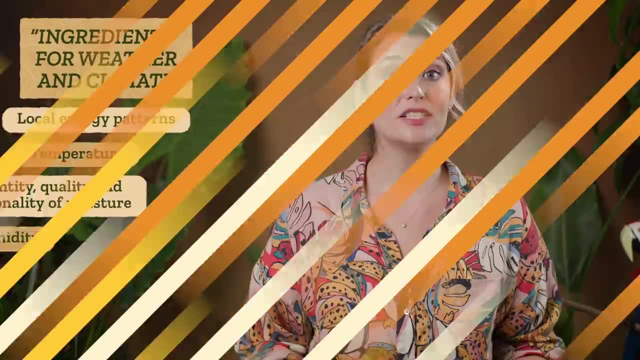 with different climates and ecological niches, which is where certain plants can thrive but not others, And they passed this knowledge down over generations, using their geographical understanding to select plots of land. Even today, farmers all over the world need to think about geoliteracy. 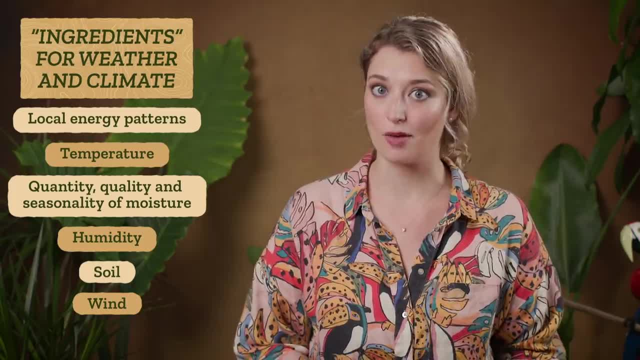 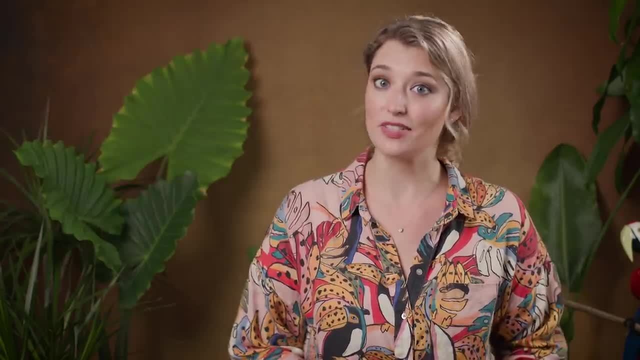 They need to think through all the ingredients for weather and climate to plant crops, And we have all sorts of technology to help them track air pressure, precipitation levels and more. But ancient Andean farmers didn't have these same tools. Let's go to the Thought Bubble. 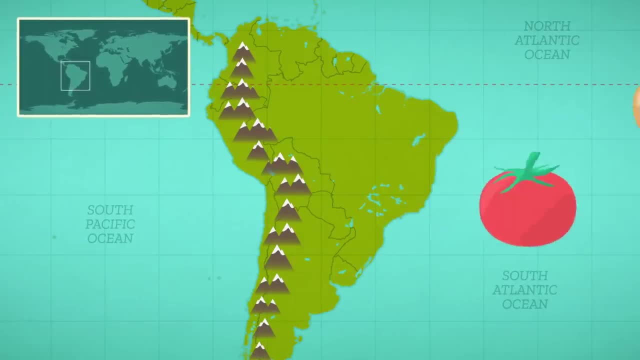 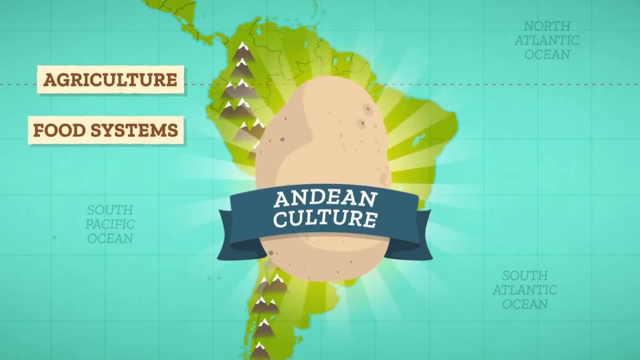 The Andean foothills and mountains are used to grow lots of crops like tomatoes, beans and maize, But the diversity of potatoes is a source of pride and a cultural symbol of traditional Andean agriculture. food systems, history, community and identity. 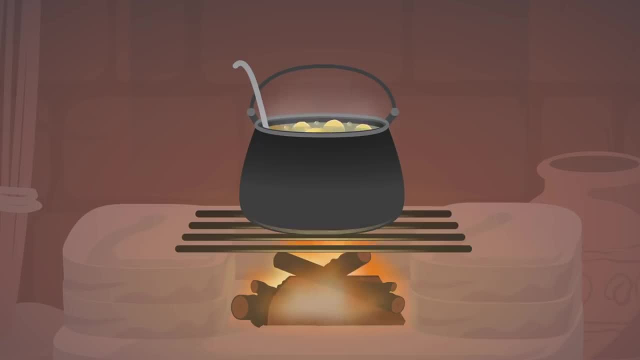 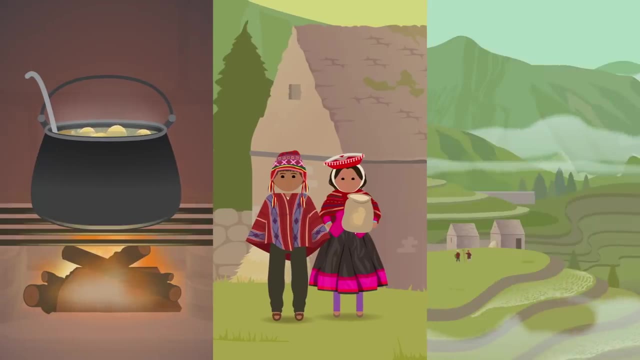 Historically, we think one way time was measured here was by how long it took to cook a pot of potatoes. Even today, potato seeds can be gifted to young couples setting up a household, And farmers in the high Andes measure land based on the area a family needs to grow their 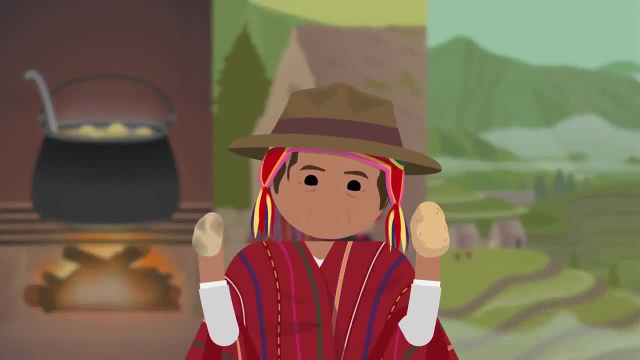 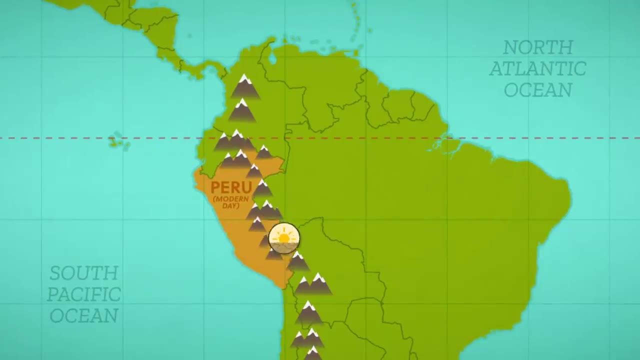 supply of potatoes. Over the years, farmers realized that when they plant, their crops could make a difference between a good harvest and a poor one. For example, areas in what's now southern Peru are prone to periods of drought. As modern geographers, we know that typically there are cold water currents along the Peruvian. 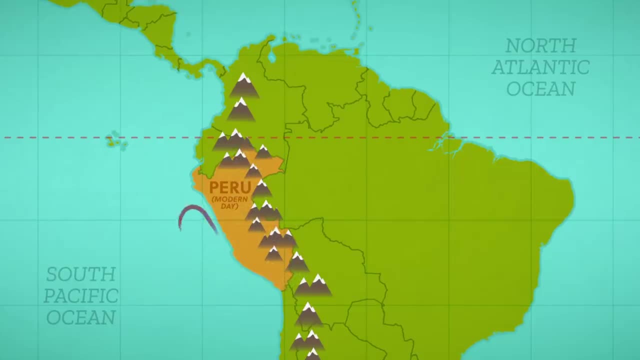 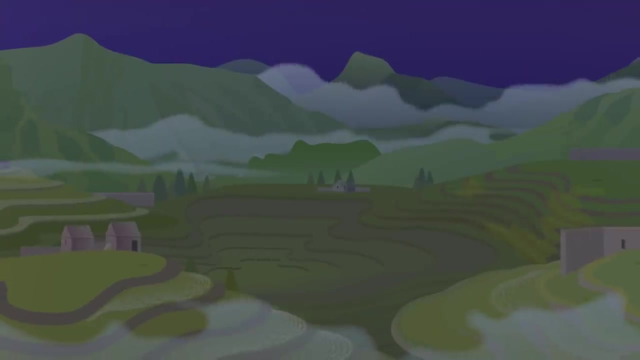 coast, which help bring rain to the Andean highlands. But some years there's a pooling of warm water along the Peruvian coast which can bring drought until the ocean currents are gone. Without the aid of satellites or an understanding of ocean currents, Andean farmers began to 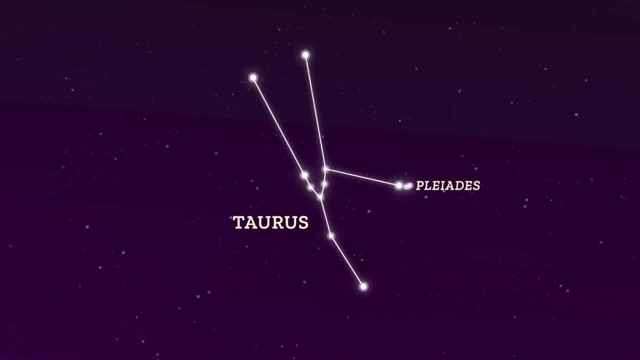 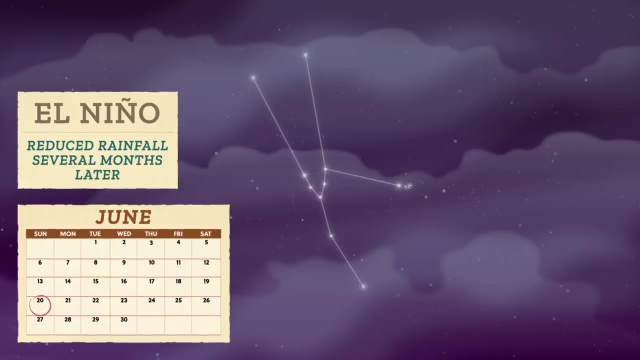 notice that if the stars, especially the Pleiades stars in the Taurus constellation, were hidden by water vapor in the atmosphere and hard to see around the winter solstice in late June, it indicated an El Niño year, which is linked to reduced rainfall several months. 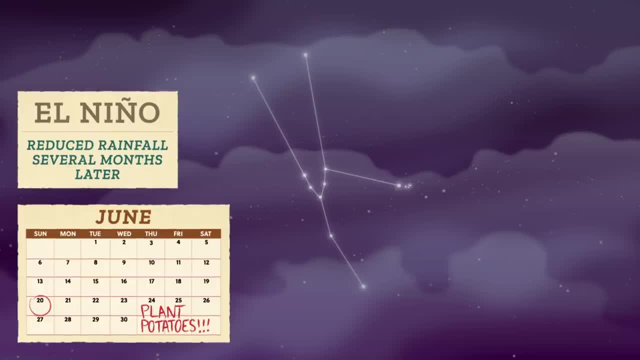 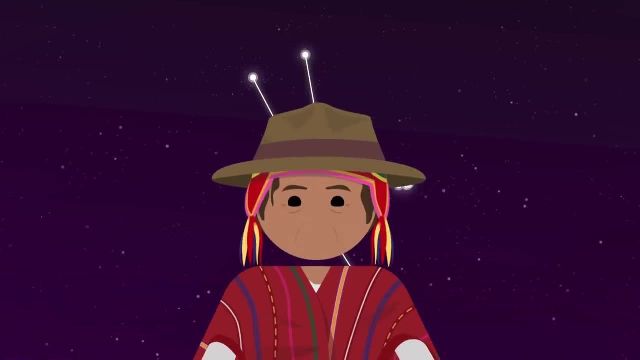 later. So they'd plant their potatoes earlier to take advantage of whatever rain that fell. If they could see the stars clearly, they knew they'd get enough water to plant the potatoes a little later. Basically, Andean farmers were geographers who observed the relationship between clouds. 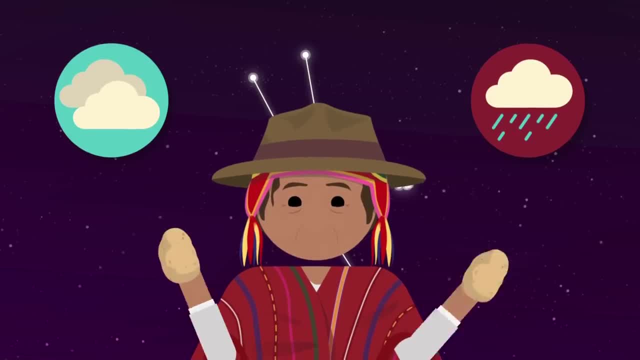 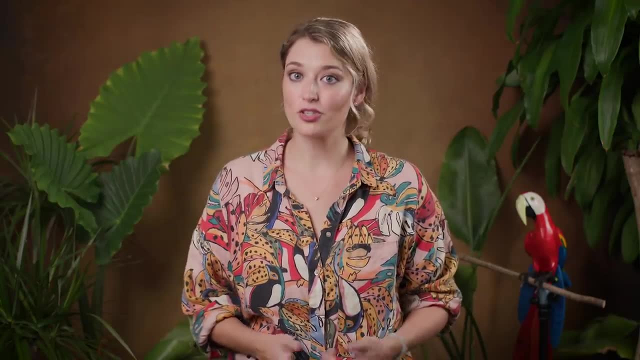 in the atmosphere and rainfall patterns later in the season, which, in turn, helped people survive in the Andes for centuries. Thanks, Thought Bubble. Any way that people observe atmospheric conditions, find patterns and make decisions based on those patterns is geography in action. 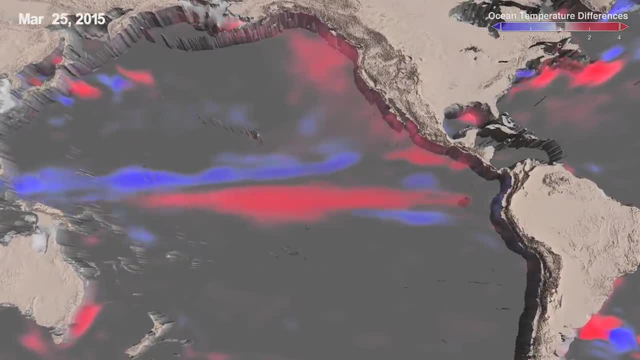 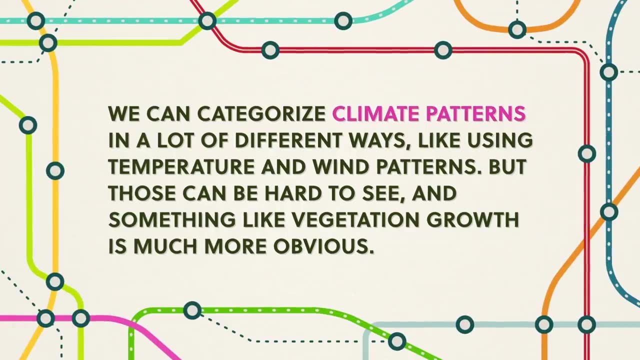 Nowadays, scientists can observe and predict climate phenomena on a global scale, from ocean current patterns like El Niño and the Southern Oscillation to what latitudes different plants like potatoes can grow at. We can categorize climate patterns in a lot of different ways, like using temperature. 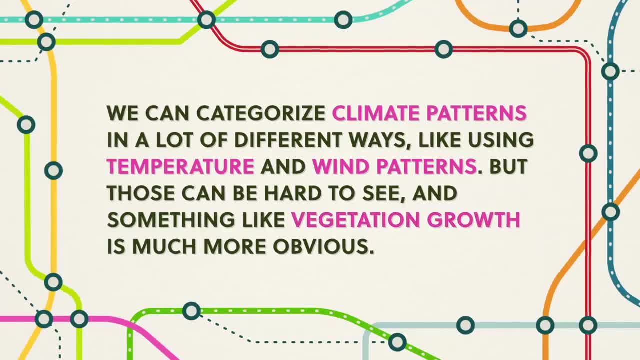 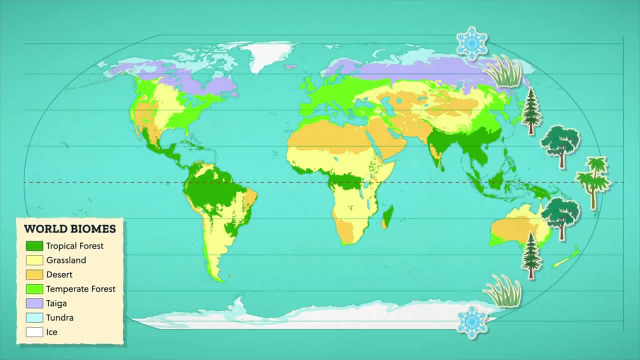 and wind patterns, But those can be hard to see. In general, natural vegetation starts with a tropical rainforest at the equator and transitions into ice and snow and sparse vegetation as we get to the poles, sort of mirroring the mountain climate pattern we talked about before. 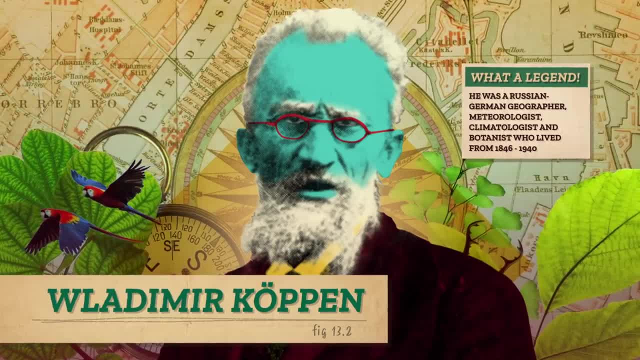 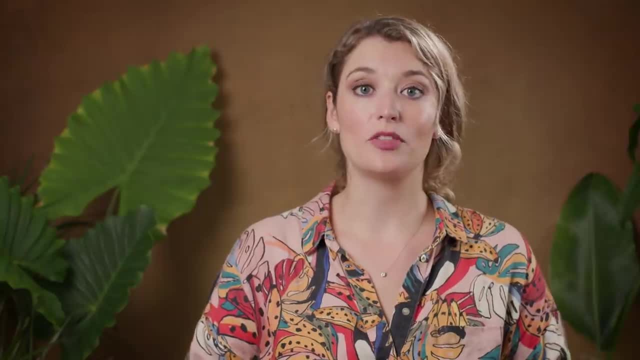 This visible connection between vegetation and climate helped climatologist and botanist Vladimir Koppen devise a classification system in the early 1900s called the Koppen system. It's still widely used today, with many improvements by many people and with many terms that reference. 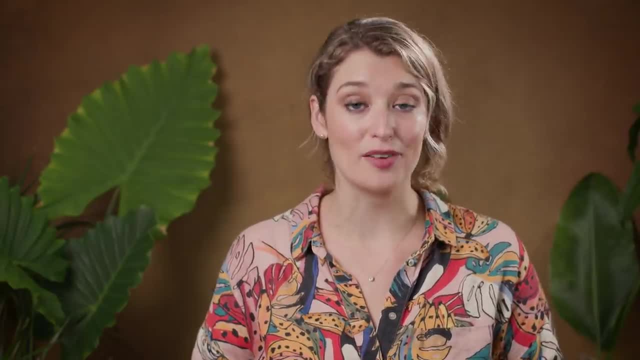 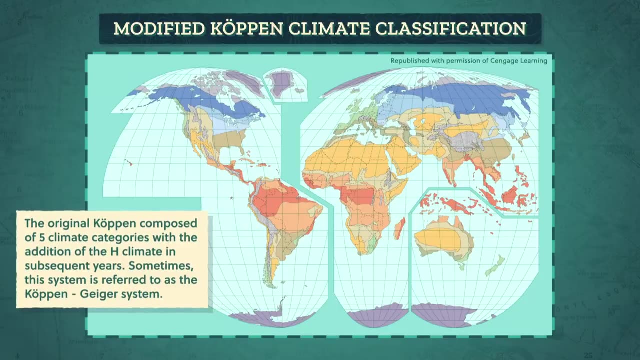 a type of climate and type of natural vegetation, like the tundra or the rainforest. Specifically, the Koppen system divides the world into six major climate categories. Using the visible vegetation as a guide, Koppen came up with precise definitions for each. 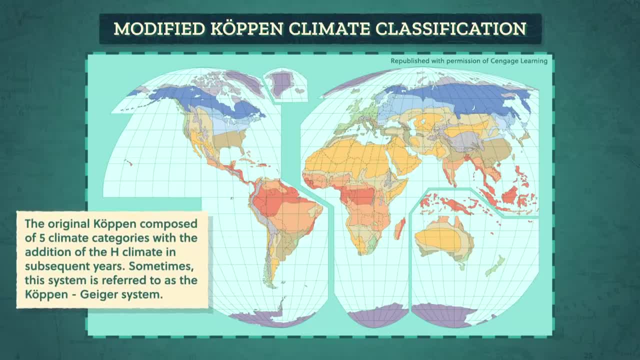 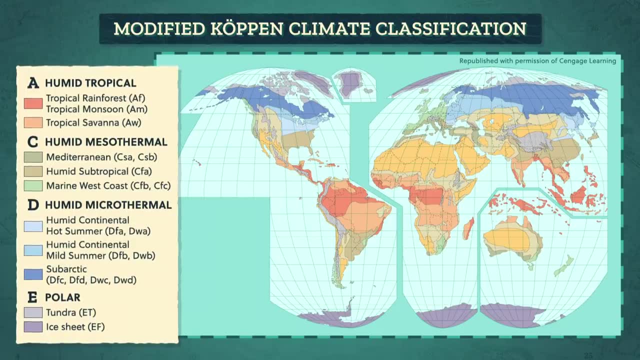 climate region based on average monthly temperature, average monthly precipitation and total annual rainfall. The first four categories are based on moisture and temperature characteristics and they're usually labeled with capital letters Like. A represents tropical climates, which are known for having high temperatures and. 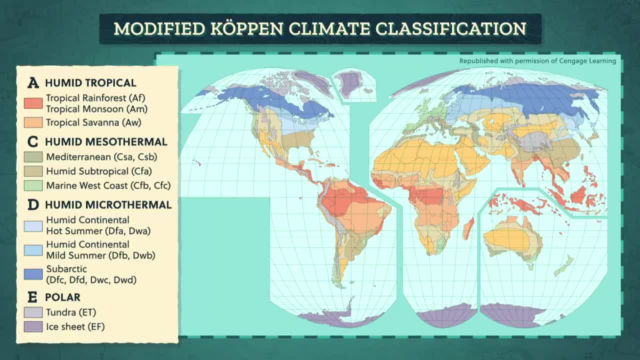 receiving a lot of rain, And E represents polar climates which tend to be cold and dry. Then the last two categories are based on temperature and temperature characteristics, and they're usually labeled with capital letters. They're also based on moisture and elevation instead of temperature. 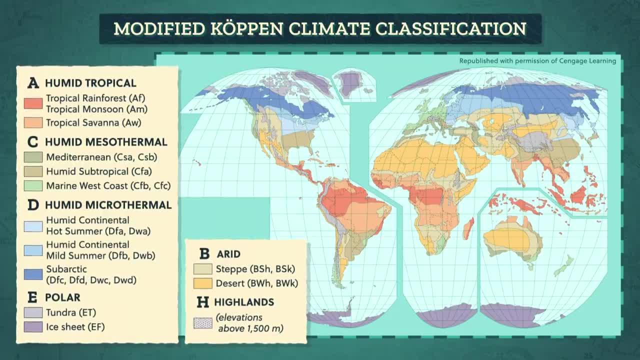 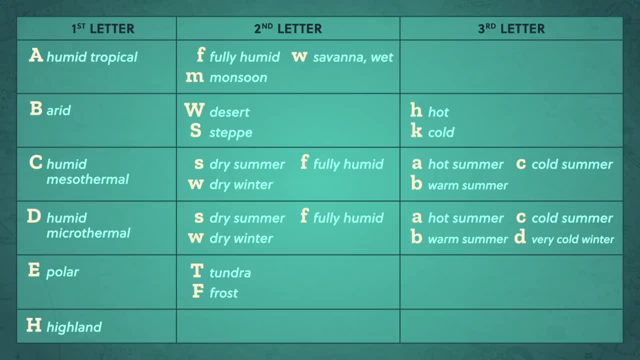 Like H represents the highland climates in the world's mountainous regions, Like where our original Andean farmers grew potatoes. Then within each of these big categories, there are subcategories marked with additional letters to break climate ups into even more precise groups. 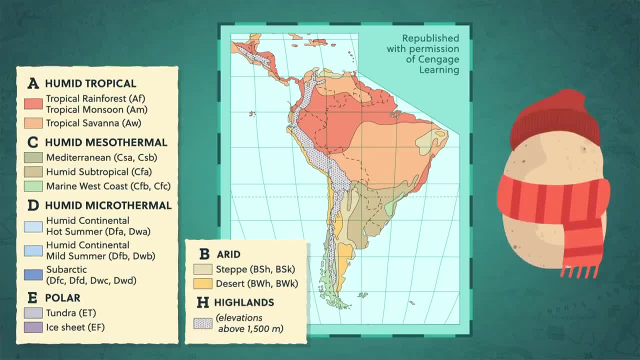 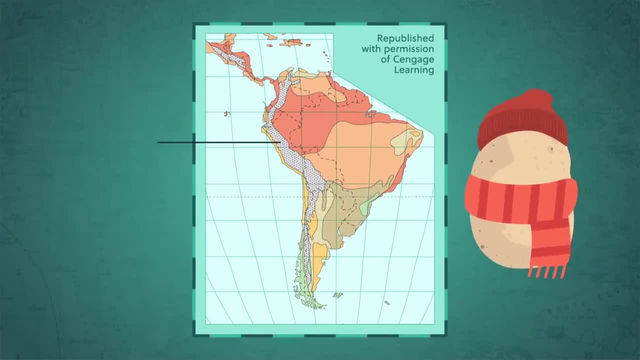 So let's use potatoes as our example. They thrive in cold weather. so if we look at a Koppen climate classification map of South America, it makes sense that they thrive in the Andes. In the west, along the Andes, there are bands of H, which means highlands, and BWK, which 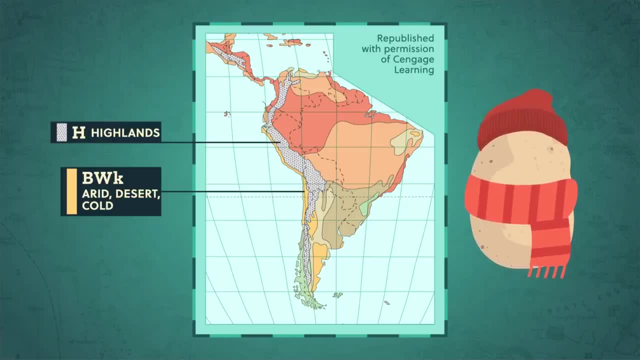 says the area is airy. In the east there's arid, desert and cold. The transition out of those desert highlands is BSK, which says the area is arid, has a steppe climate and is cold. Those are some ideal potato growing conditions. 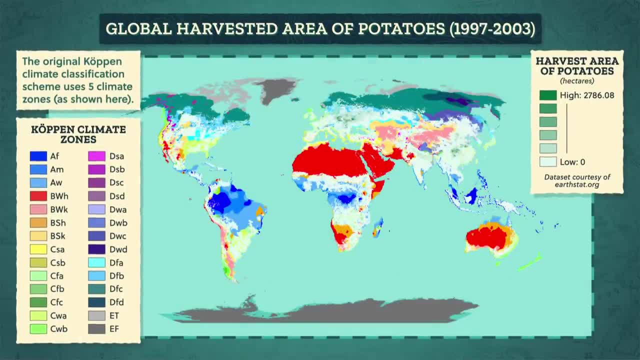 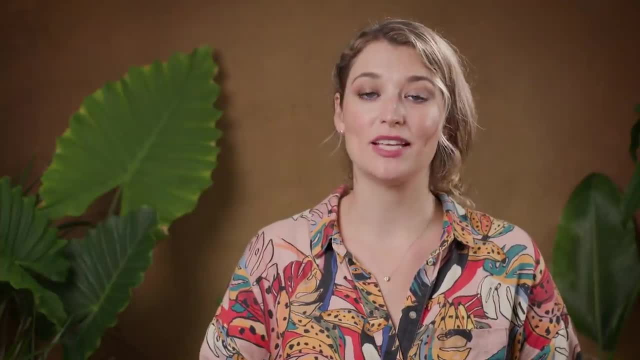 If we overlay a full Koppen climate classification map with a map of everywhere potatoes are grown, we see that potatoes are really hardy because there's a lot of overlap with different climates. We know that many species of potato were domesticated by Andean farmers, but we also know that plants 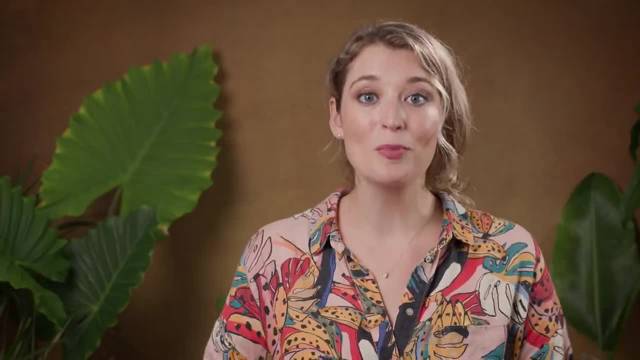 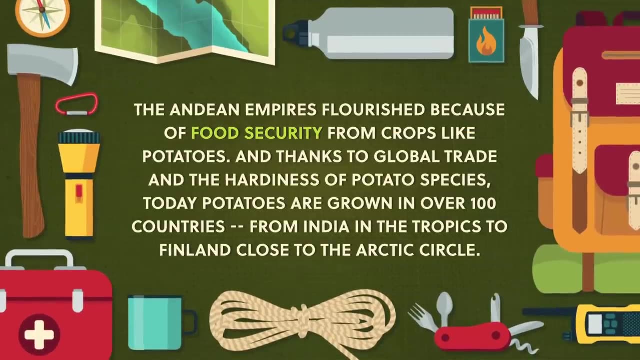 are adaptable. Those farmers used their geoliteracy to grow more plentiful crops, but also to begin breeding. So if we look at the map, we see that potatoes are hardy. They're not breeding plants to tolerate different temperatures. The Andean empires flourished because of food security from crops like potatoes. And thanks to global trade and the hardiness of potato species. today potatoes are grown in over 100 countries, from India, in the tropics to Finland, close to the Arctic Circle, From hot and cold regions to dry and wet regions and all climate combinations in between humans. 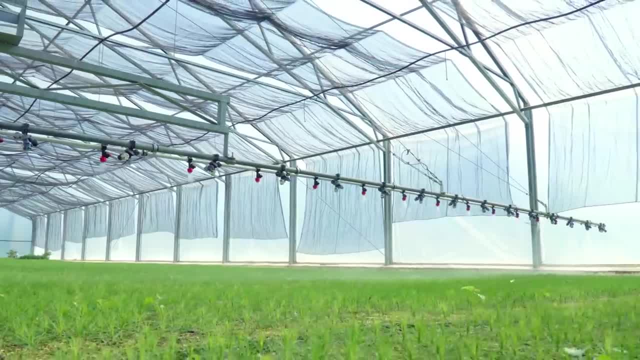 have adapted to the natural environments around us and used our growing geoliteracy to thrive, But increasingly the Earth's environments are also impacted by our choices. In future episodes we'll look at how potato crops are adapted to the natural environment of the world. 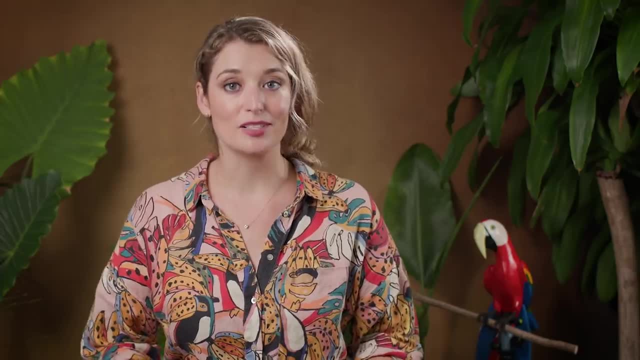 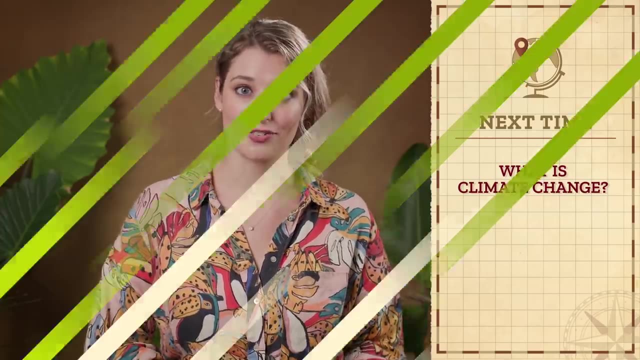 We'll look at how and why maps of global climates, vegetation, soils and ecosystems are changing and our response to those changes, And we'll hit the ground running in the next episode when we discuss how these themes relate to climate change. 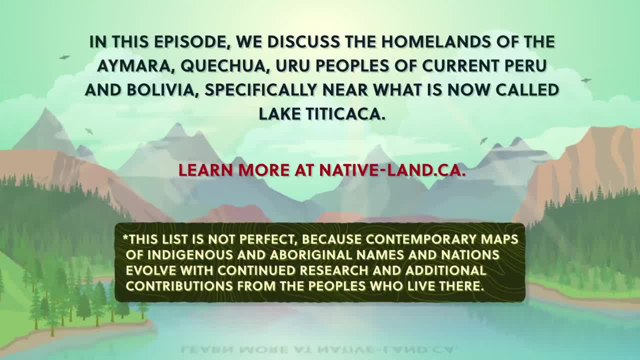 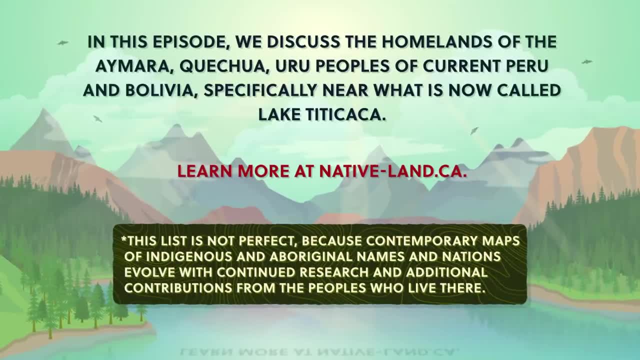 Many maps and borders represent modern geopolitical divisions that have often been decided without the consultation, permission or recognition of the land's original inhabitants. Many geographical place names also don't reflect the indigenous or aboriginal peoples' languages. So we, at Crash Course, want to acknowledge these peoples' traditional and ongoing relationship. 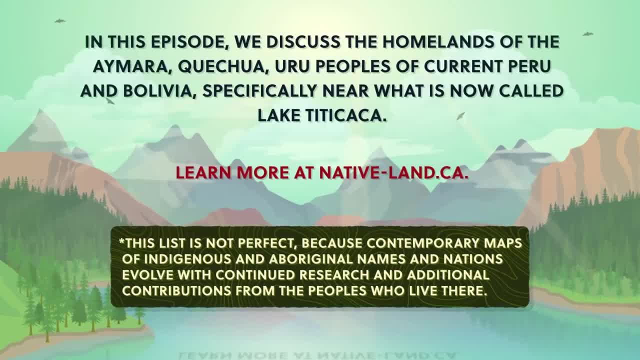 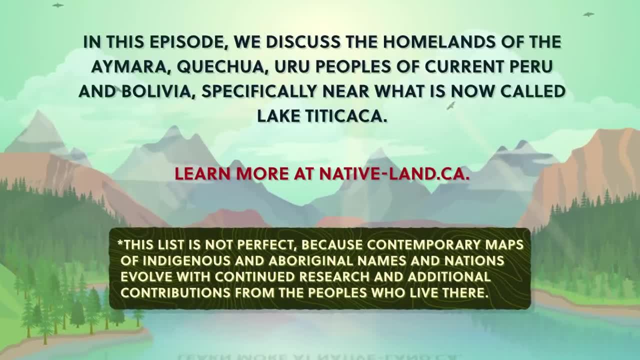 with that land and all the physical, cultural and cultural aspects of it. We encourage you to learn more about the history of the place you call home through resources like native-landca and by engaging with your local, indigenous and aboriginal nations through the websites and resources they provide. 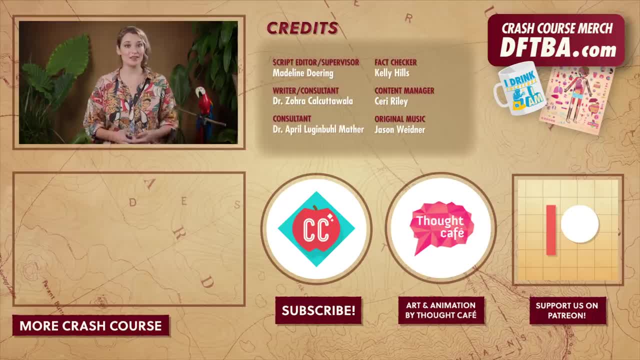 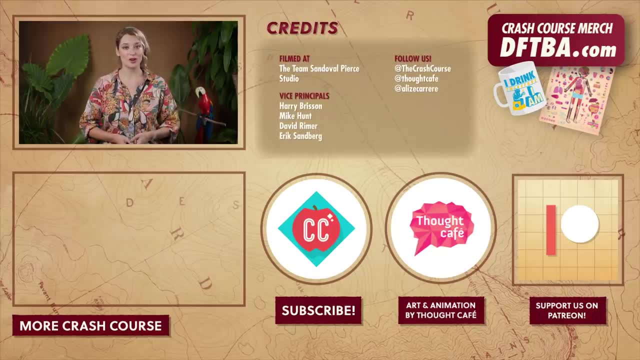 Thanks for watching this episode of Crash Course Geography, which is filmed at the Team Sandoval Pierce Studio and was made with the help of all these nice people. If you want to help keep Crash Course free for everyone forever, you can join our community.